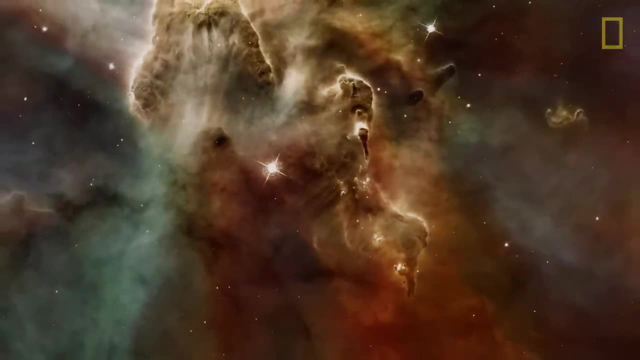 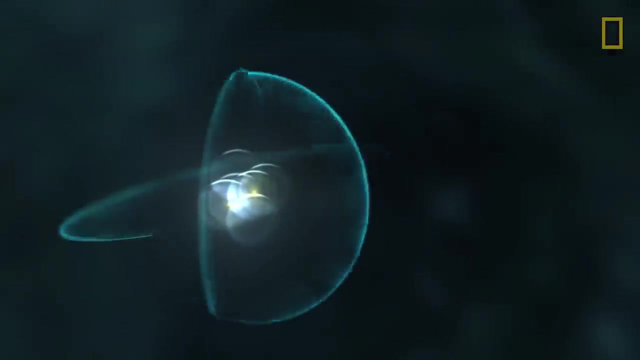 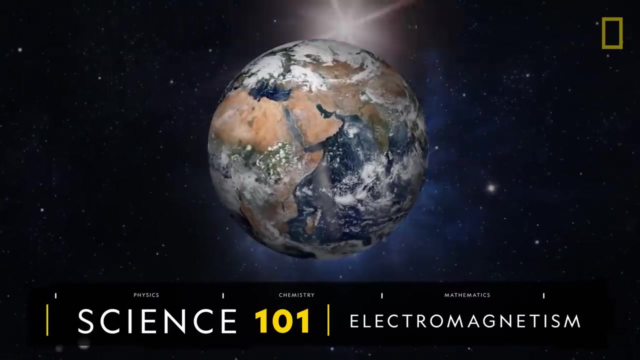 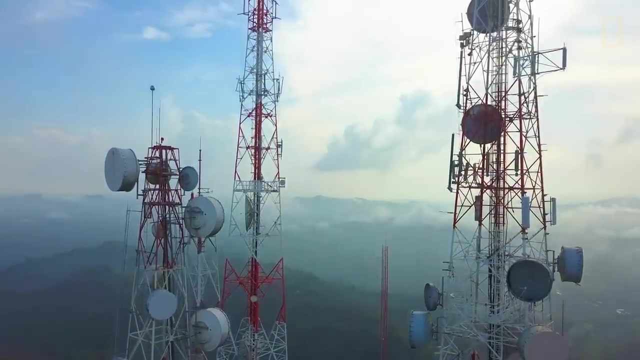 Electromagnetism, or the electromagnetic force, is one of the four fundamental forces of nature. It generates light and energy and holds atoms, matter and the world as we know it together. Electromagnetism is a branch of physics that studies the interactions between electric and 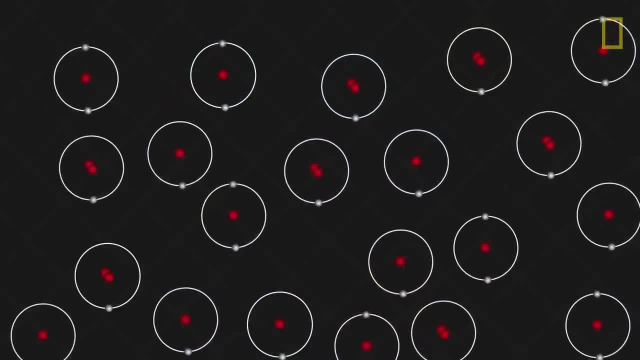 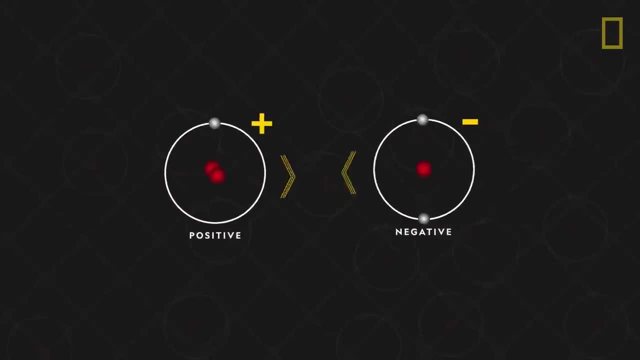 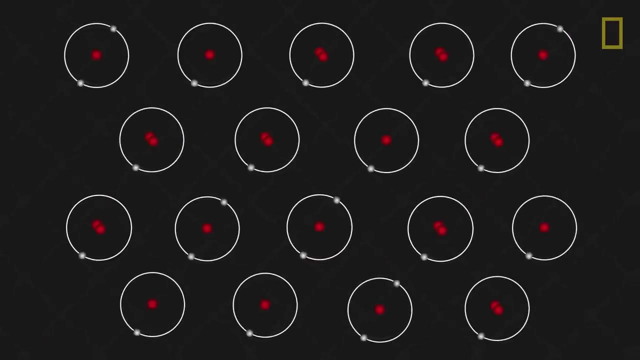 magnetic fields. All matter has an electric charge, which can be positive, negative or zero. Opposite charges attract, while like charges repel. These electric forces bring and hold atoms together. and when atoms gain a positive or negative charge through the transfer of electrons, 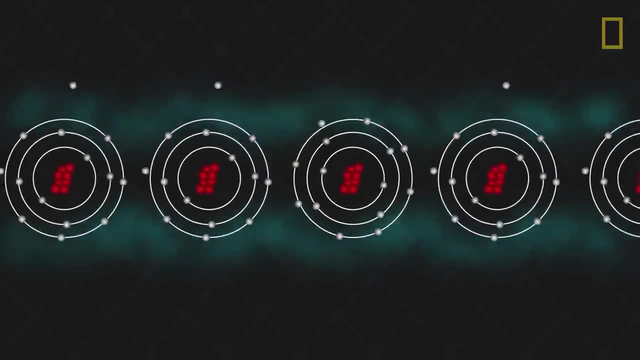 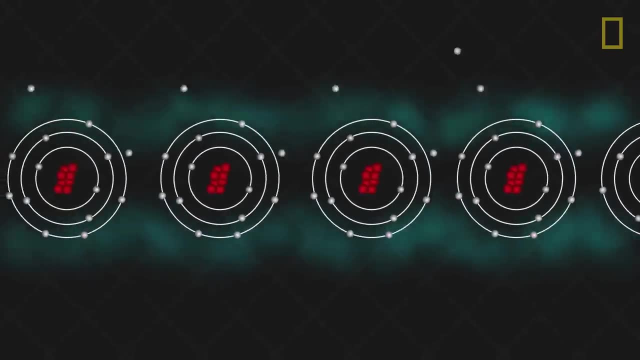 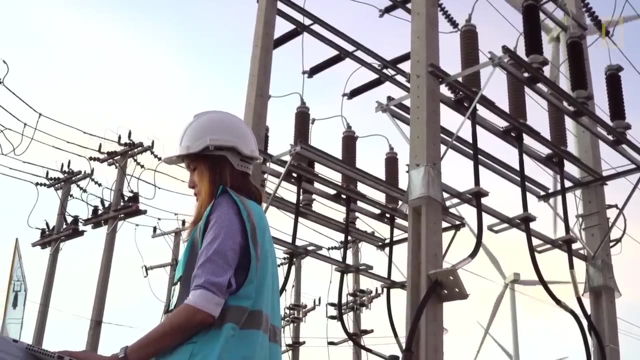 a measurable electric field will form. If those electrically charged particles start to move, the field will become a flowing electric current and form a magnetic field around it. Under the right circumstances, interacting electric and magnetic fields can continuously produce and sustain one another. 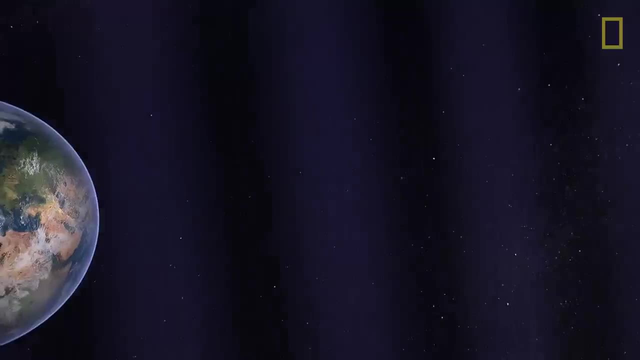 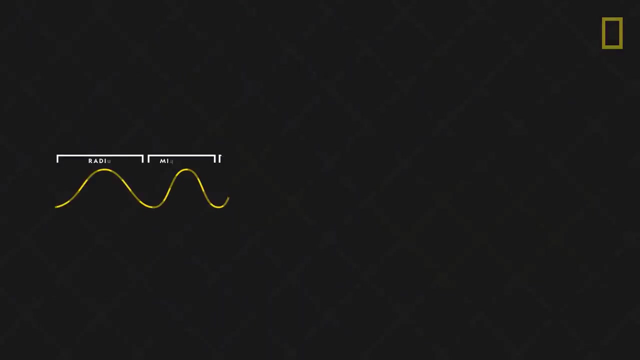 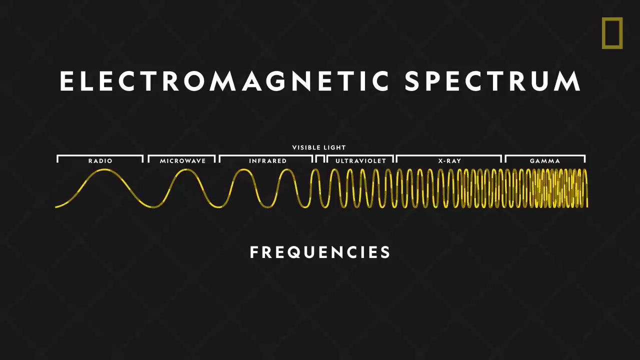 This generates an electromagnetic field that transmits waves of electromagnetic energy or radiation into space. The intensity of this radiation is determined by its frequency. These frequencies make up what's known as the electromagnetic spectrum. Near the middle of the spectrum is visible light, such as light emitted by stars. 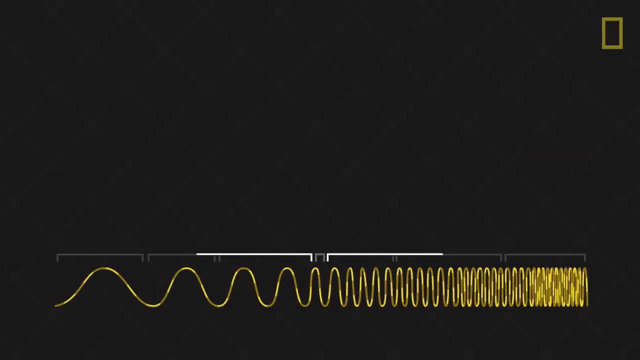 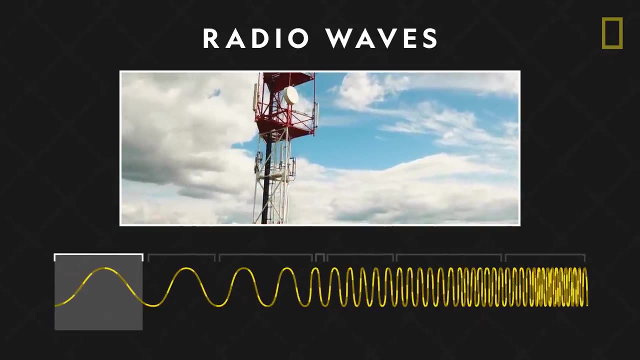 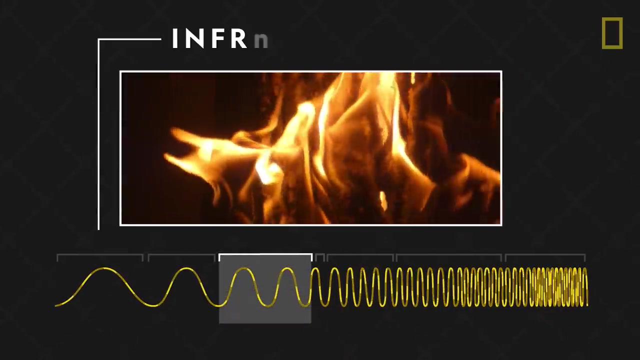 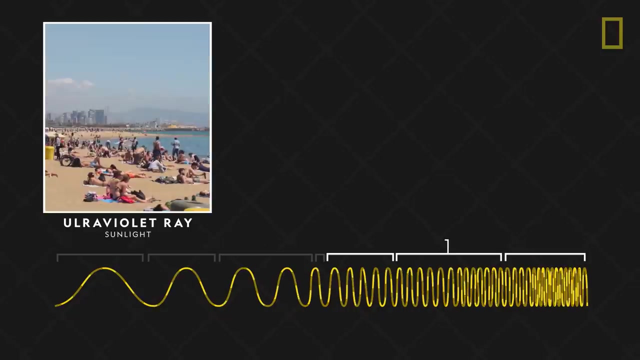 fireflies and computer screens. On either side are invisible electromagnetic waves. On one end are long low-frequency radio waves that broadcast television and radio signals, microwaves that carry telephone signals and cook food, and infrared waves emitted by fires. On the other are short high-frequency wavelengths, ultraviolet X and gamma radiation. 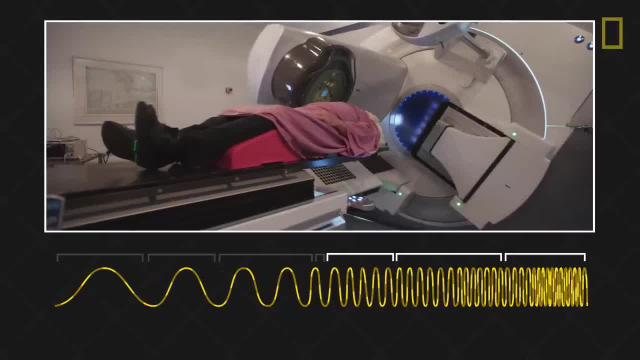 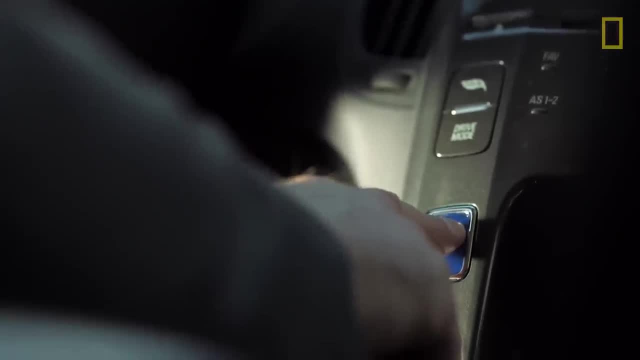 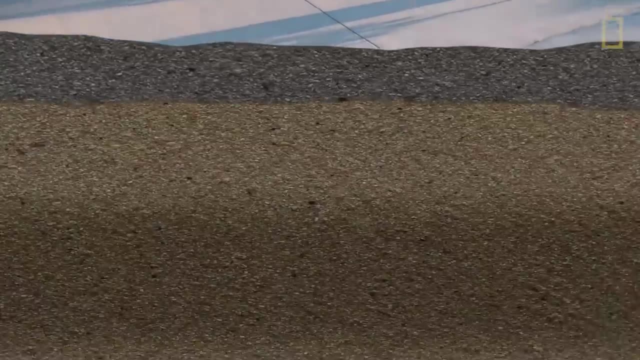 Unlike low-frequency waves, these waves can pass through the human body, making them useful for medical applications. While electromagnetism has daily applications, it's also the engine that drives the planet as a whole. Thousands of miles below the Earth's surface, a layer of liquid metals.